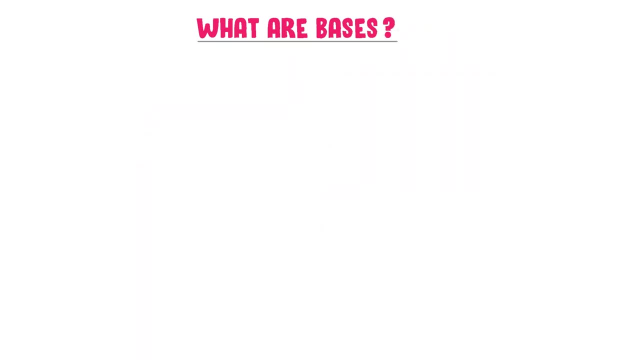 Now, what are bases? Well, bases taste better. And they are also found in many substances which we use in our daily life. For example, 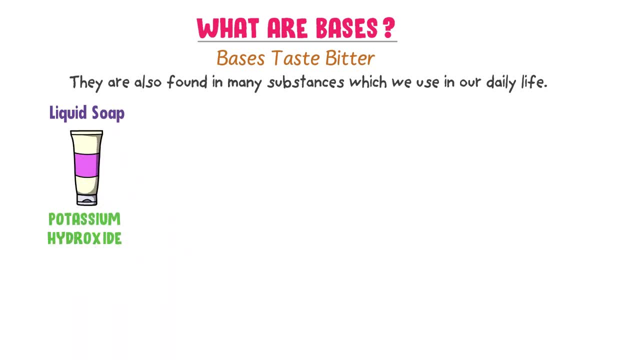 liquid soap. It contains potassium hydroxide. Secondly, baking soda. It contains sodium bicarbonate. 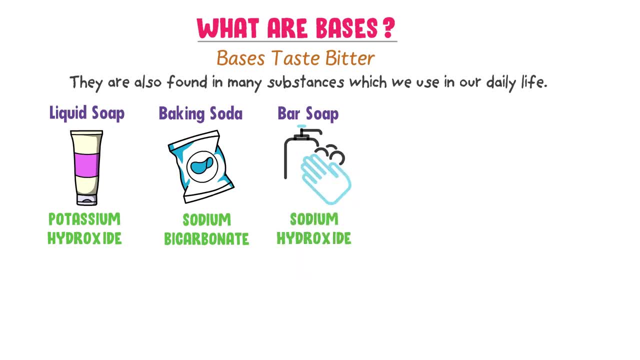 Thirdly, bar soap. It contains sodium hydroxide. Fourthly, detergents. They contain ammonia. Fifthly, washing powder. 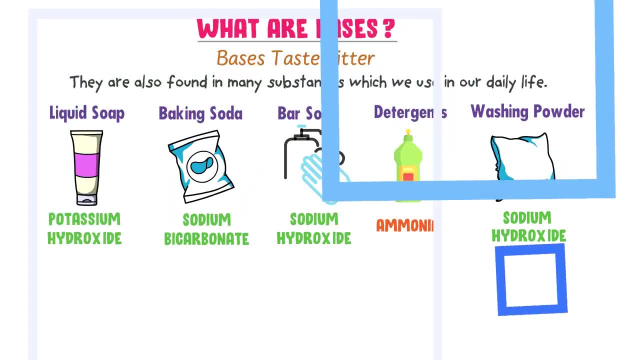 They contain sodium hydroxide. So, different substances contain different bases. 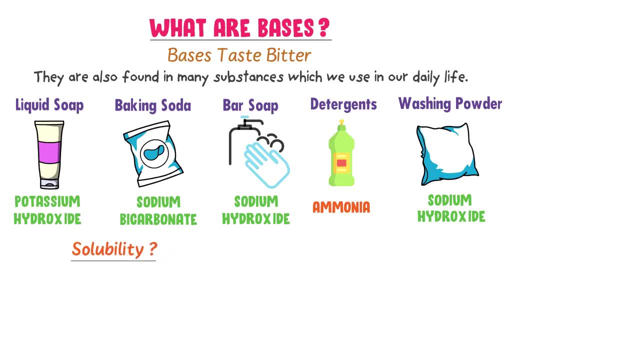 What about the solubility of bases? Well, some bases are not soluble in water. Bases that are soluble in water are also called alkalis. 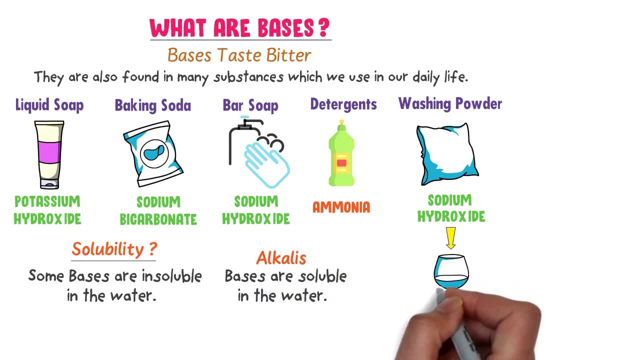 For example, sodium hydroxide in the soup is soluble in the water. So, sodium hydroxide is a base as well as alkali. 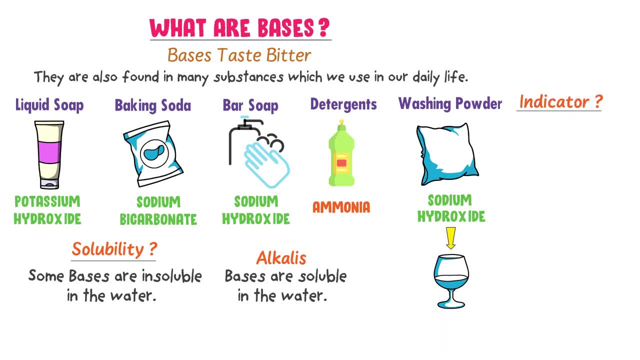 Now, what about the indicator test of bases? Again, we can use different indicators to test the presence of bases. 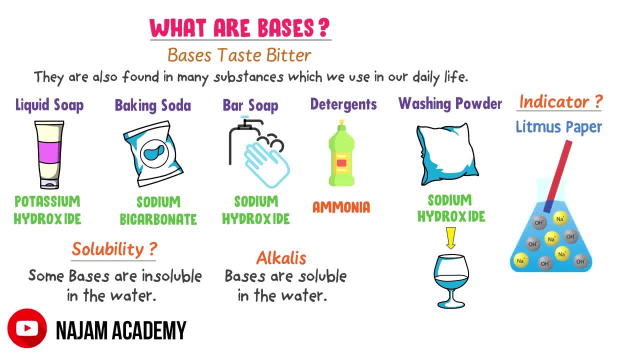 But the simple test is litmus paper. Bases turn red, litmus paper blue. 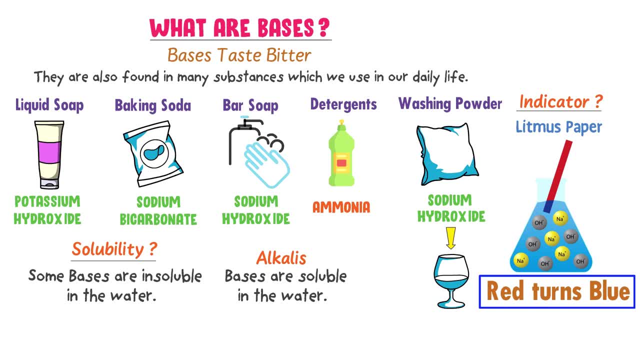 Let me repeat it. Bases turn red, litmus paper blue. 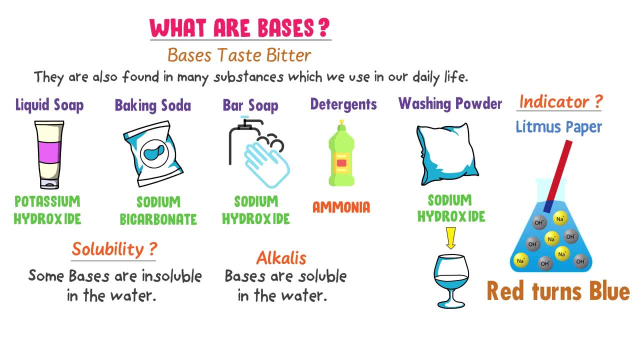 Thus, remember that bases taste bitter. Different substances which we use in our daily life contain different types of bases. 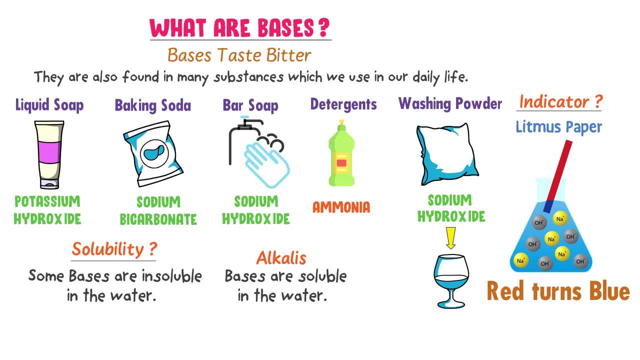 Bases that are soluble in water are also called alkalis. And bases turn red, litmus paper blue. 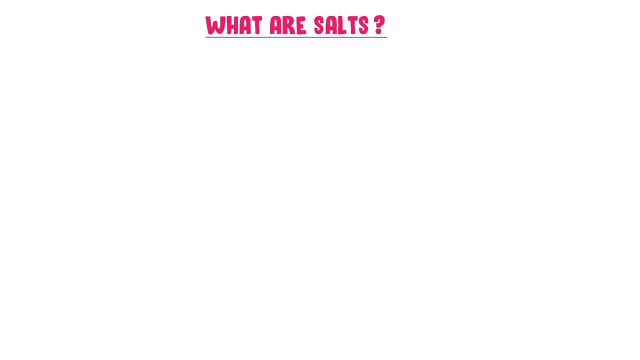 Finally, what are salts? Well, salts taste like this. Salts taste salty. 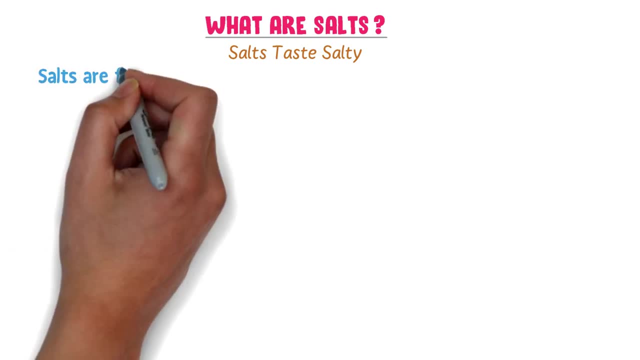 But different salts may taste different. Salts are formed and the neutralization reaction of acids and bases.